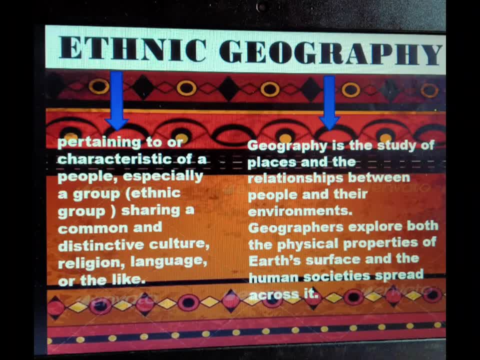 So geography is the study of the places and their relationship towards the people who are living in it, and also their environment. I do believe that geography was further and deeply explained by our first reporters. Okay, so let's go now. So what is ethnic geography? 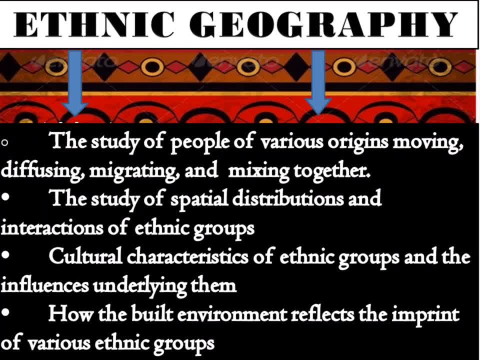 Okay, so ethnic geography is the study of people of various regions moving, diffusing, migrating and mixing together. It is also the study of spatial distributions of interactions of ethnic groups, cultural characteristics of ethnic groups and the influences underlying them and how they build. 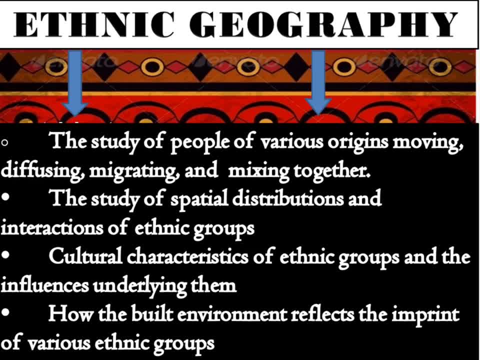 And it includes diffusing or migrating. It also includes interaction. So, in short, geography or ethnic geography is the study of human interaction and their environment. so, um, according to jimmy buffet, he said that without geography, you are or we are nowhere, which is true because, um, geography or ethnic geography takes us. 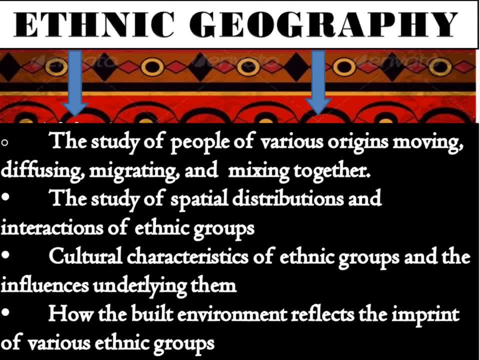 to step further, to know further our roots. so some of the questions answered by ethnic geographies are where the the group of people settled, which is incorporated with that group, where, where did they came from, um, why did they leave their old home? and, lastly, why did they choose? 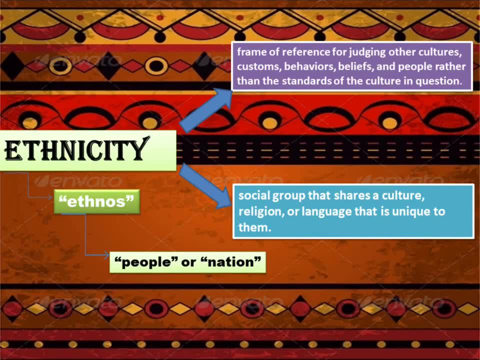 this place to settle specifically. okay, so to know further, what is ethnicity? let's see. so ethnicity is, or came from the word ethnos, which means people or nations. so ethnicity comes with a group, so it is a group of certain people, because people is plural and not singular form, so it is therefore a group. so ethnicity is a frame of reference for judging. 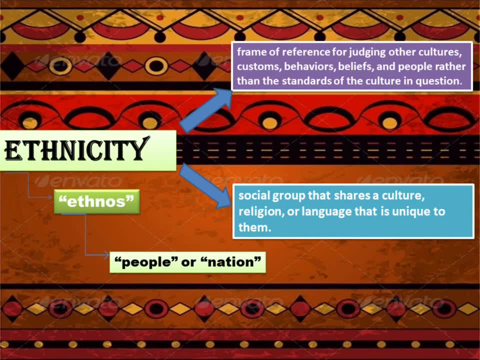 other cultures, customs, behaviors, beliefs and people, rather than the standards of the culture in question. so social group: it is a social group that shares a culture, like mentioned earlier before, religion or language that is, that is unique to them. so ethnicity, will they call uh ethnicity as a frame of reference, because sometimes 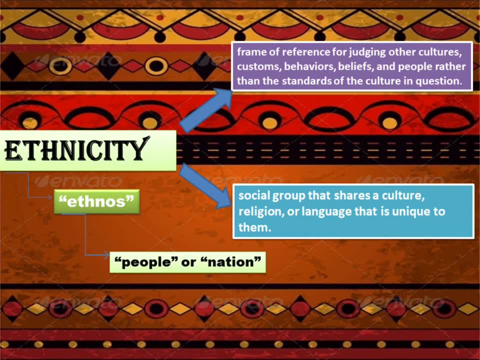 ethnicity becomes the basis of someone to judge a certain group. we sometimes, we usually- do this, which is often a fallacy, for example, when we hear the word or the ethnic group in locations. what do we know? so? in general, we know them as what they are: good in cooking peanut. 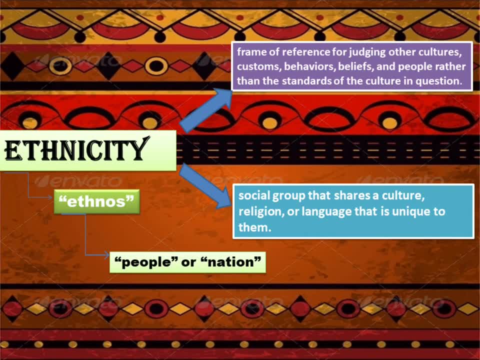 bet they are korea pot, which is what we know about the ethnic group entrances or ethnic groups maybe or not, but they are likely to be the case in terms of policy. if you see these words, i think it is a common thing. i think people in foreign countries want to have a certain group, for example, when we hear the word or the ethnic group, it might be the case of someone who is not an ethnic group, but 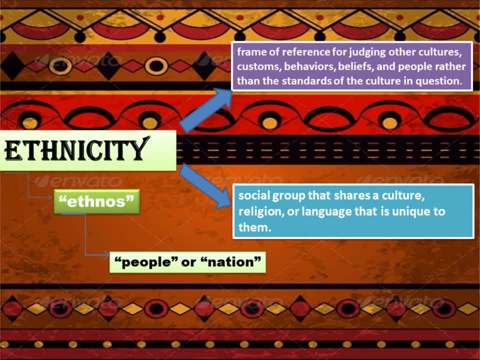 Ilocanos, but is often a fallacy. why? because, yeah, they know generally they are good at cooking pinakbet and currypot, but not all Ilocanos are a good cook of pinakbet and they are not currypot. so ethnocentrism is the feeling. 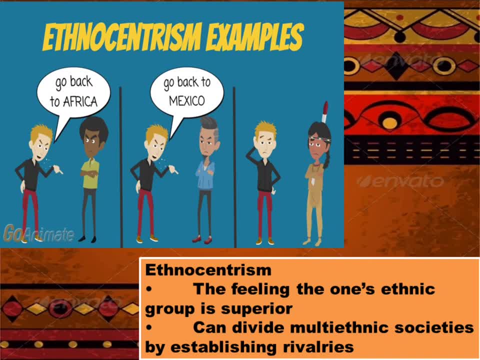 of ethnocentrism is the feeling the one's ethnic group is superior and can divide multi ethnic societies by establishing rivalries. so ethnocentrism often results. sometimes into rivalries. so ethnocentrism is the feeling that one's own ethnic group is superior than others. 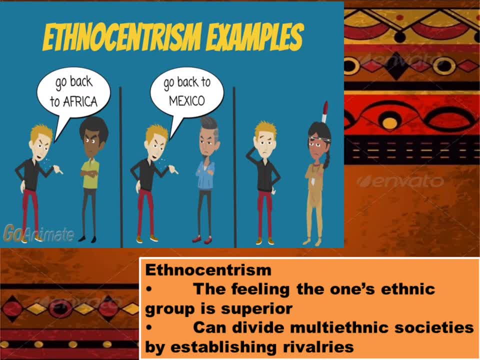 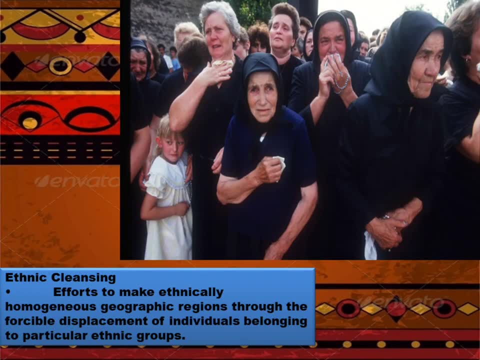 ethnocentrism is very much alive, especially in today's world. so let's go now to next ethnic cleansing. so ethnic cleansing is the effort to make ethnically homogeneous geographic regions through the forcible displacement of individuals belonging to particular ethnic group. sorry, excuse me, sorry, excuse me. 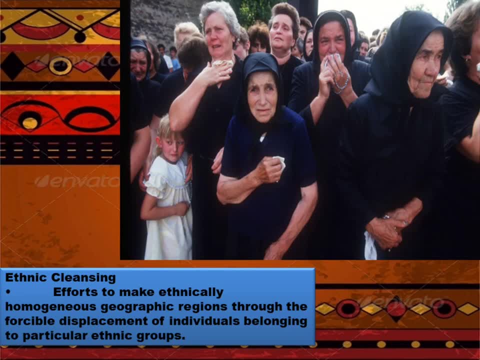 so ethnic cleansing is one of the worst. why? because it is done by force. it is usually done by force. what they do here is they force other culture to leave the area so that there will be just one ethnic group left to settle the area. so pinapa less nila you. even ethnic group the Meron's is an area a. 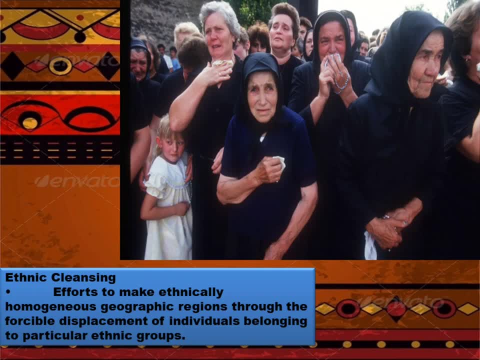 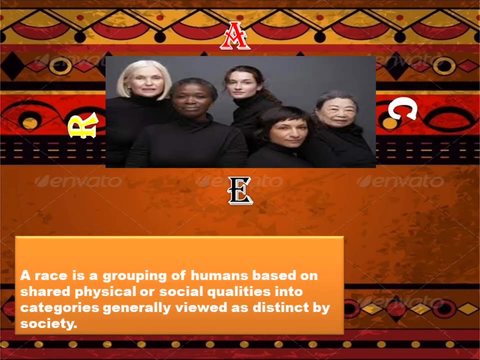 so that you will not lose, you know, at era malama's area on IE is an culture. so that is what they call, what we call ethnic cleansing, which is totally worst. the race is a group of humans based on shared physical or social qualities in to categories generally viewed as distinct by society. 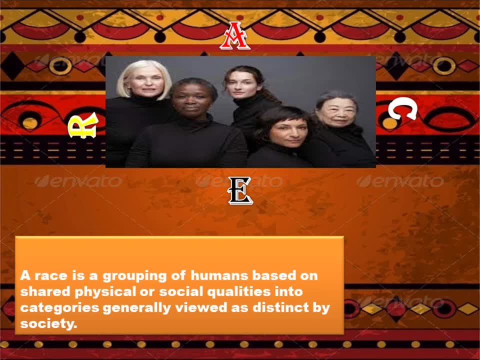 So sabi dito. it's a group of human based on shared physical or social qualities. Meaning physical, it talks about our physical features or physical attributes. So race is often understood to be similar with ethnic, But race is genetic. 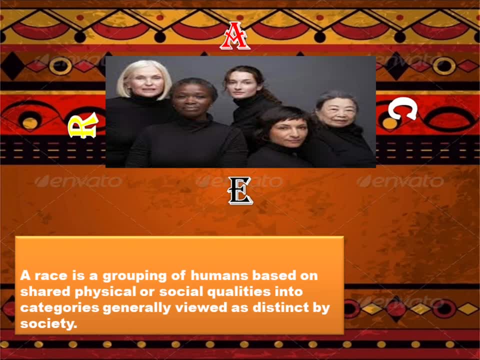 It talks about our physical features, like our hair, the color of our hair, eyes, the shape of eyes, skin tone and others. It is biological, because it is passed through generation to generation, through gene, because it is hereditary. So hereditary siya. 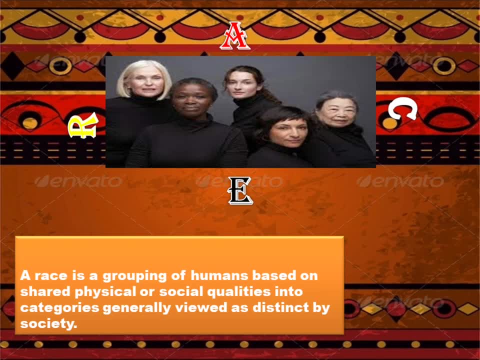 Meanwhile ethnic. Ethnic is culture. Let me just explain this, because yun nga napag alamang ang race at ethnic ay isa, but no. So race is a shared physical feature, Meanwhile ethnic is a culture. So it is and can therefore be learned. 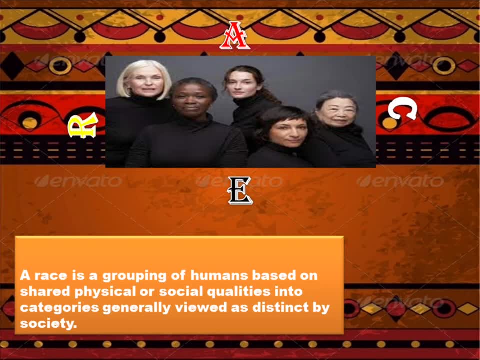 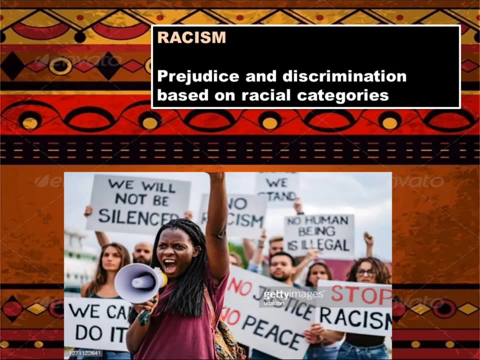 So that is the difference between race, And race leads to what we call racism. So what is racism? Racism is a prejudice and discrimination based on racial categories, And this is very much alive in today's generation. So pag sinabi natin yung racism, the best and the usual and common illustration of racism is racism. 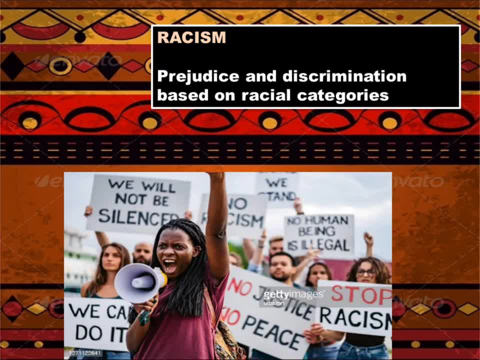 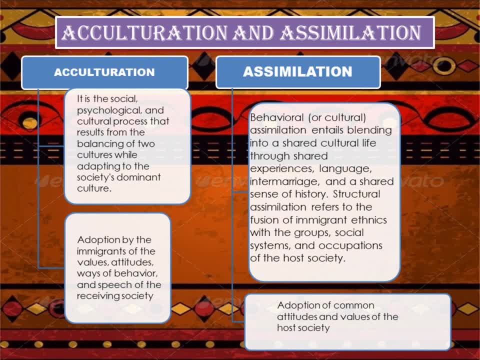 So pag sinabi natin yung racism the best and the usual and common illustration of racism is racism Acculturation, It is the social, psychological and cultural process that results from the balancing of two cultures while adapting to the society's dominant culture. 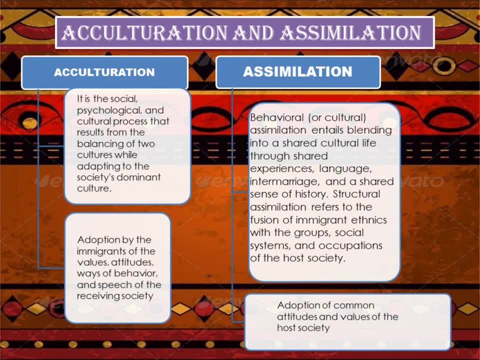 It is an adaption by the immigrants of the values, attitudes, ways of behavior and speech of the receiving society. It is an adaption by the immigrants of the values, attitudes, ways of behavior and speech of the receiving society. so acculturation is the. 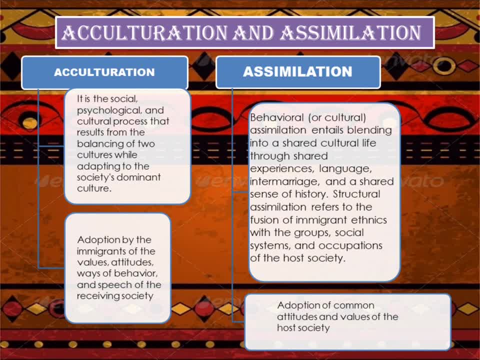 adaption, so it is adapting to the dominant culture or, if ano, yung majority ng ethnic group sa lugar na pinuntahan mo, dun ka susunod. for example, if I go there in Baguio City, since I am from lowland, I am from 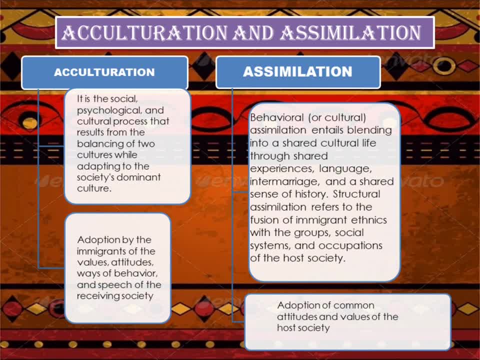 Kirino, as mentioned, and I go to Baguio, which is Thailand. I should adapt to their culture, pero managing pa din yung culture na kinalakyan ko or yung culture na meron ako, which is the culture from the region to which is. 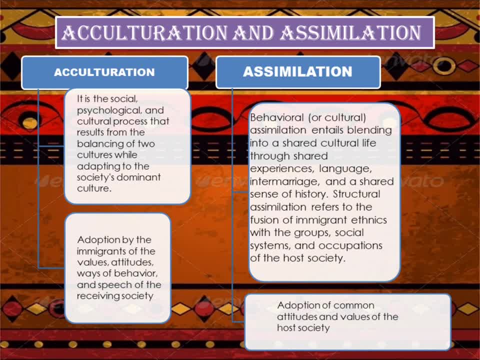 Kirino. so meanwhile, assimilation- assimilation is a behavioral or cultural assimilation entails blending into a shared culture life through shared experience, language, intermarriage and a shared sense of history. structural assimilation refers to the fusion of immigrant ethnics with the group's social systems. 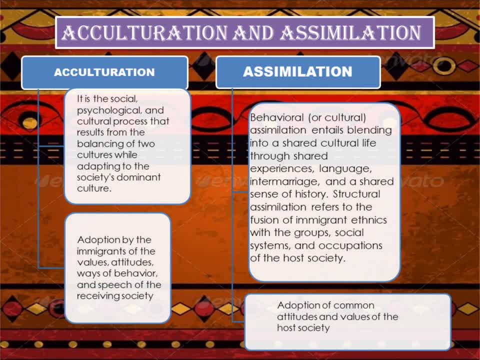 and occupations of the host society. so it is also an adaption of common attitudes and values of the shared or the host society. so it is also an adaption of culture趣, of their own culture and culture. but assimilation does adopt the culture of the dominant. 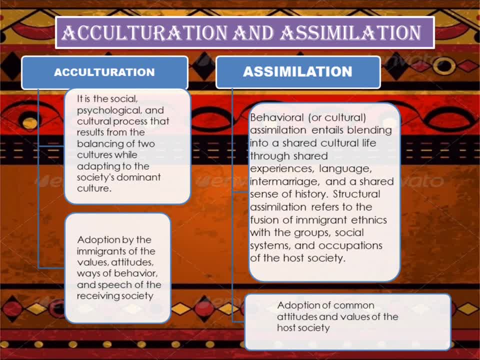 culture, but that manages to balance his or is her own culture. but also, but assimilation is the total blending or the adoption of common attitudes or culture and values of the host society. so we have to live with their culture. the perfect example is like what was was mentioned merrily. 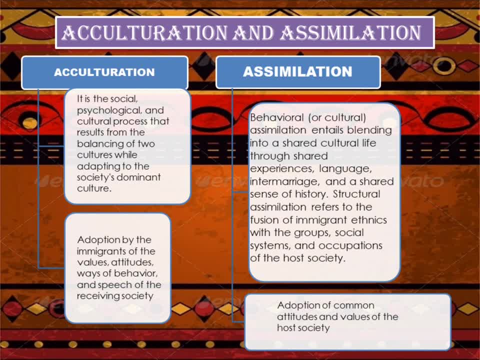 last year, the idea that this culture leads to indifference in, For example, the wife is an Ilocano and the husband is Igorot. In the Philippines, we still follow patriarchal culture, So what mostly happens is that the couple will live in the husband's place. 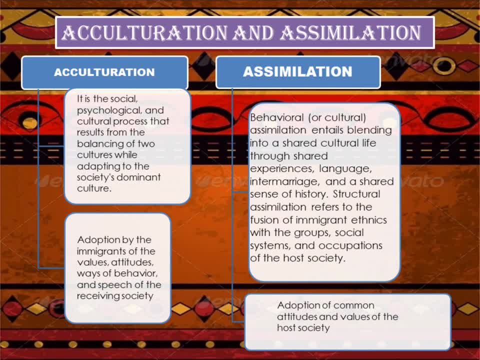 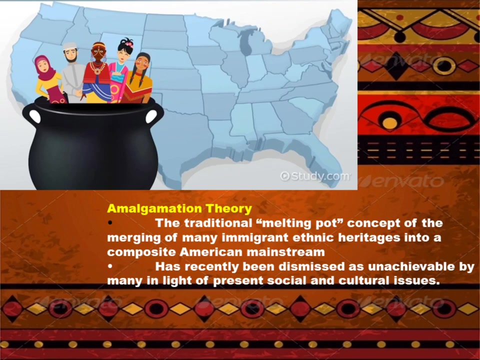 where the wife needs to adapt her husband's culture so that she can blend in. So that is the difference between acculturation and assimilation, Though the adoption is both needed in the two processes. but they have that difference. You can see in the picture. we have here a pot and a different group of people. 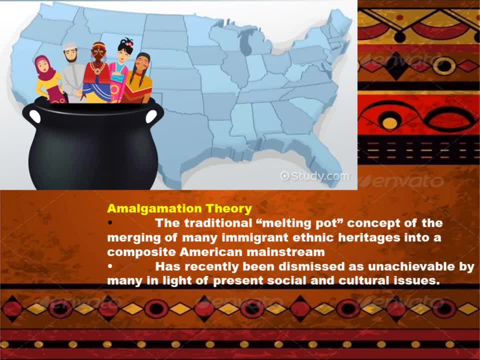 Or let's say different ethnic groups, So what We call this, the amalgamation theory, or the traditional melting pot concept of the merging of many immigrant ethnic heritages into a composite American mainstream or into a place. So this is the name, as you can see in the picture in the pot. 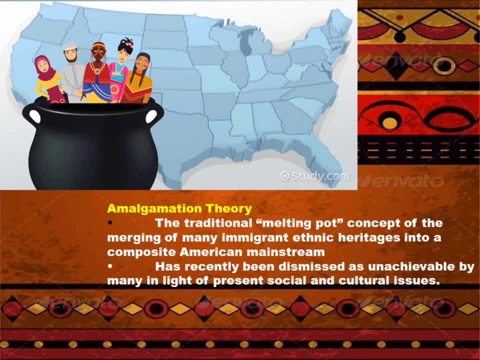 This is one pot, but there are many, There are many ethnic groups. So it says here it is a melting pot concept of the merging. So when we say merge, for example in the spreadsheet in Excel, when we have columns, we can merge that and the two cells will become one. 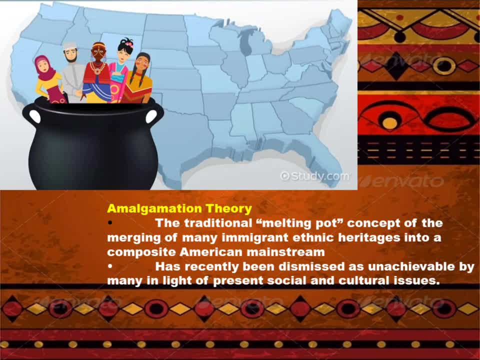 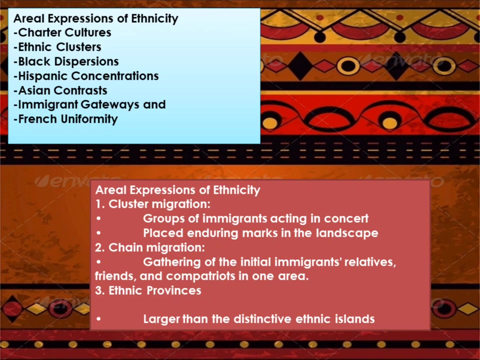 So here this is the combination of different ethnic groups So that it can form one. So it has recently been dismissed as unachievable by many in light of present social and cultural. So let's go now to the next. So we have here aerial expression of ethnicity. 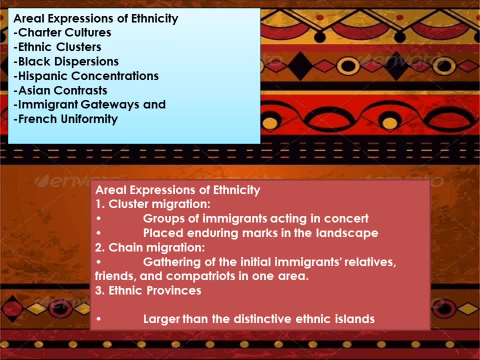 So charter, first of all charter cultures. When we say charter culture, we are talking about a group of people. When we say charter, it refers to the policies created to cultures in order for it to be manageable. So this is for cultures. 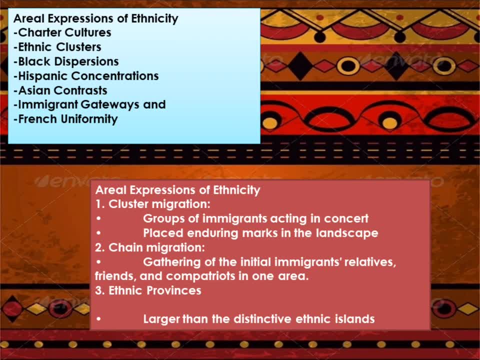 Next, we also have ethnic cluster. Ito ay, ito ay ang pagpapangkat-pangkat ng ating mga pangkat etniko, So another aerial expression of ethnicity. We also have here the black dispersion, Sorry. 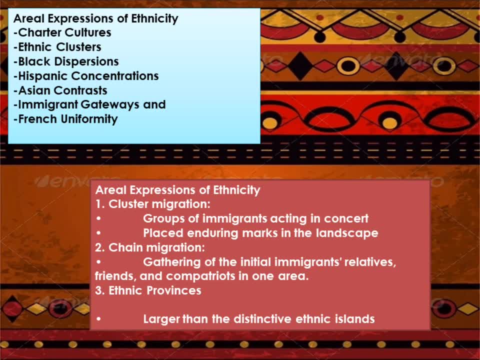 So when we say black dispersion, this is so much present in the United States of America, where they disperse blacks para maging isahan na lang Yan. So example of black dispersion is the emancipation following the civil war. Blacks engage in sharecropping and farm labor. 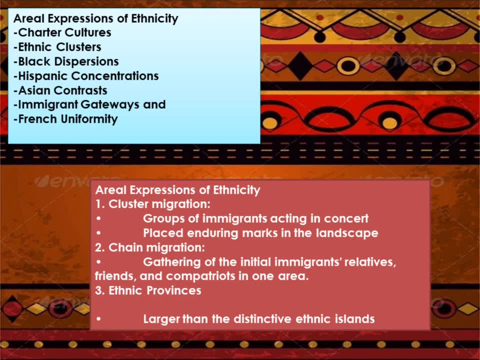 So dito na-de-degrade yung mga rights ng mga blacks, Kasi nga in US we know that na before talaga yung discrimination against blacks is very rare. So next, Asian contrast, Asian contrast. Most probably Asian contrast, it is the Asian versus Western or from the other regions of other regions of the world. 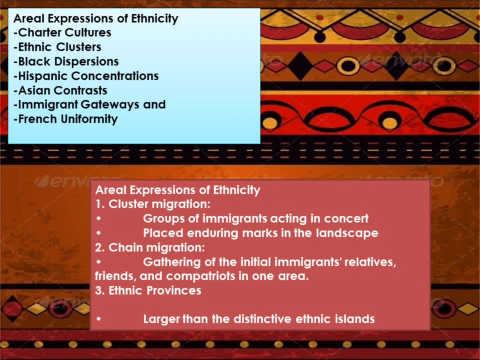 So ito yung discrimination against us Asians. So naging sikat to sa TikTok, which is the TikTok trend. Where Asian are you? So yun nga Another. immigrant gateways and French uniformity, So French uniformity, ito naman yung mga sa French. 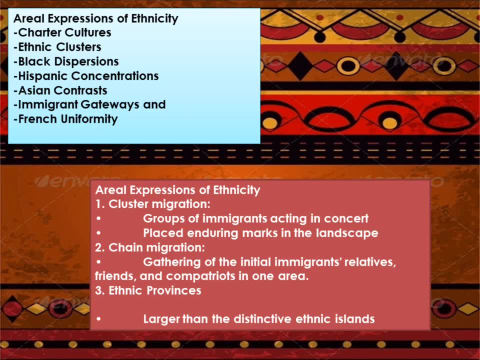 So probably sa Europe na ito. So another tagdag ko lang sa Asian contrast. So example of the Asian contrast is that the family reunification became an immigration policy in 1965. Which there Asians take the full advantage of it. 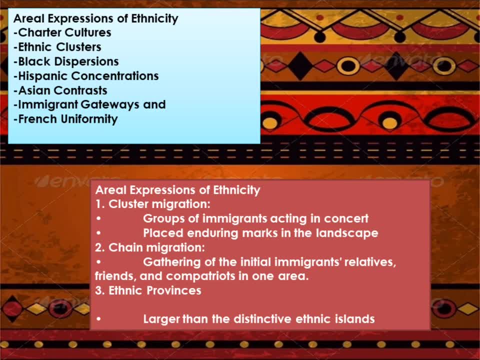 So let's go now to the aerial expressions of ethnicity. Number one: the cluster migration. So when we say cluster migration, it is where groups of immigrants, acting in concert, So place enduring marks in the landscapes. Eto, it is the many people move at once as a group. 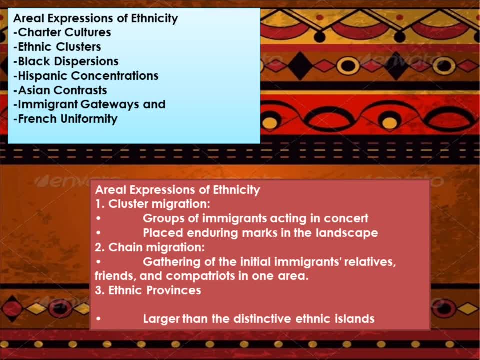 So ibig sabihin it is a kind or a type of migration Where a group, where they migrate as a group, So group sya Halimbawa dito sa amin as a barangay, as a group or as a barangay, magmamigrate kami into another barangay. 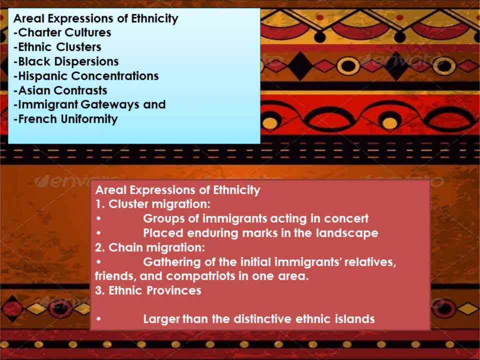 So that's it. Another example also is the Europeans in Canada and the Mormons in Utah. So next migration, we also have chain migration. So it is gathering of the initial migration, relatives, friends and compatriots in one area. So it is the assembly in one area of relatives, friends, attracted by the first settler's reports. 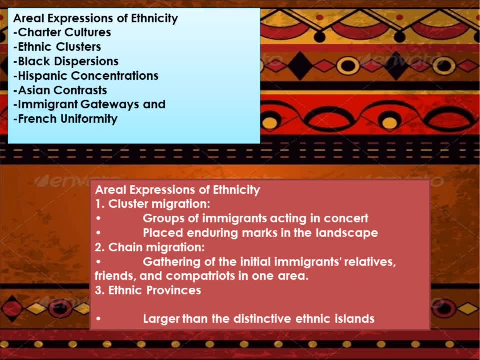 So maybe yun nga sabi. dito it is the assembly in one area of the relatives. Kung sa cluster migration kanina as a group sya nagmigrate, dito naman is the relatives Halimbawa ako pupunta, ako sa US. 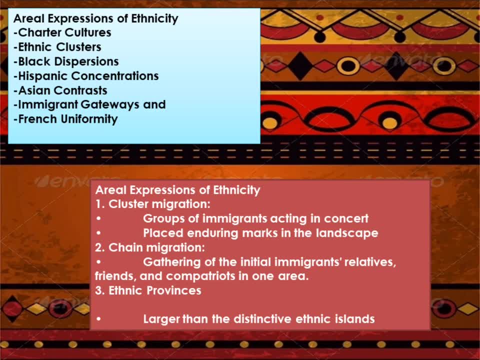 And madaming opportunity doon. So tatawagin ko ngayon yung mga relatives ko, wherein susunod din sila. Like mostly ng relatives ko, susunod din sila. Like mostly ng relatives ko, susunod din sila. 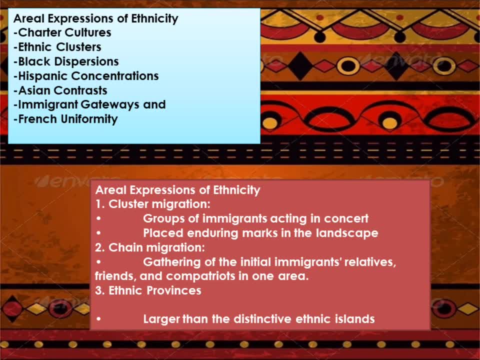 That is an example of chain migration. So next one: we have the ethnic province. Larger than the distinctive ethnic islands, It is a large number of ethnic minorities to have settled in a region. So Ito naman hindi na siya basta-basta. 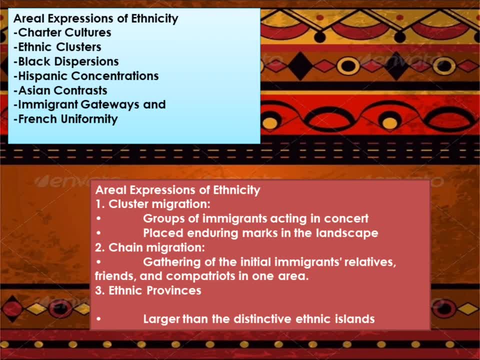 basta. basta, hindi na siya. basta, basta, group, so group siya. but then it is large number of ethnic sa pinag-uusapan na dito na magmamigrate ay a large number, or madaming bilang ng ethnic minorities to migrate in a province. so, for example, example dito is the blacks in the 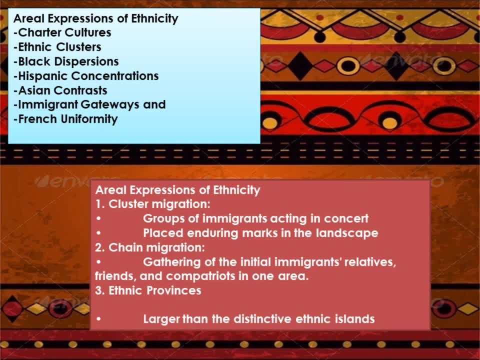 southeast, you are southeast united states, so east part of the us, or you know you mississippi and other areas. we know that mississippi was had to buy or pinning ira honey in a black black americans and he also have french canadians in quebec. so that are examples of ethnic provinces. 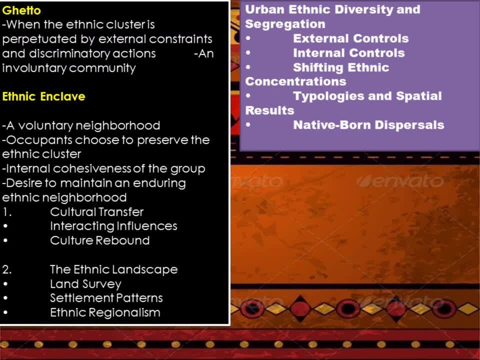 you okay. so let's now go to next. okay, ghetto. when we say ghetto, the ethnic cluster is perpetrated by external constraints, and constraints are the end discriminatory action. it is an involuntary community. so ghetto is when an ethnic community persists or persevere because outsiders discriminate the ethnic groups. so ghetto is actually a european term, a european term again that was used by first. 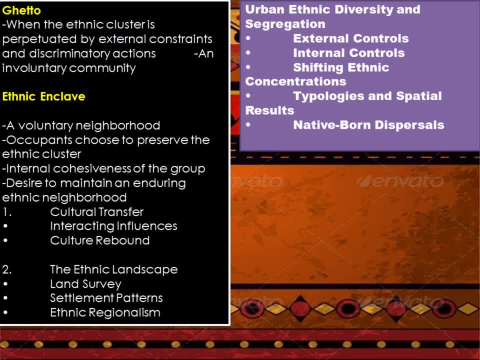 used by jews. so why do we have ghettos? it's because of racism and discrimination, like explained earlier. so we also have ethnic enclave. so ethnic enclave is a voluntary neighborhood occupation. choose to preserve the ethnic cluster. it is the internal cohesiveness of the group and the desire to maintain an enduring ethnic neighborhood. so when 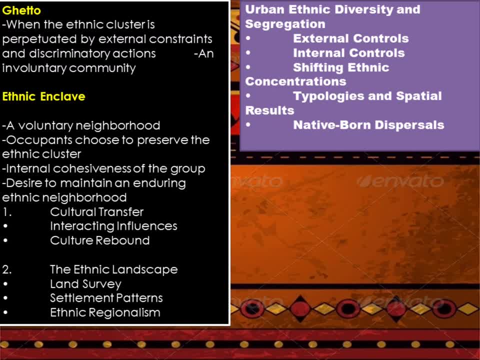 we say enclave kase. it is when an ethnic community persists or continue because the ethnic group wants it to keep, wants it to keep it to preserve. so, uh, wait, so they, they are based in order for it to preserve. number one: the cultural transfer, or culture transfer. they transfer their culture into, uh, each one, so it is the interacting. 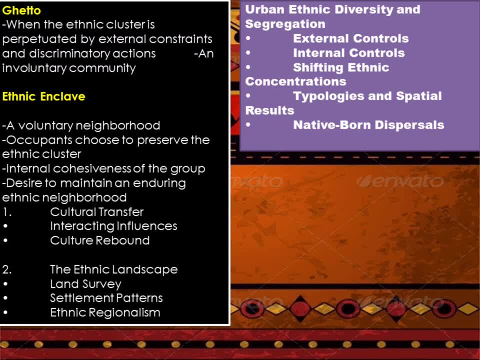 influences or culturally bounded fields, the context of the кalan, while vere, as a or no language is, or gem is used. right for it they have in order to prefer them. they prefer to pick multiple species or to have extremly different areas to. so next one, we have also the ethnic landscape: our land surveys, settlement patterns and ethnic regionalism. 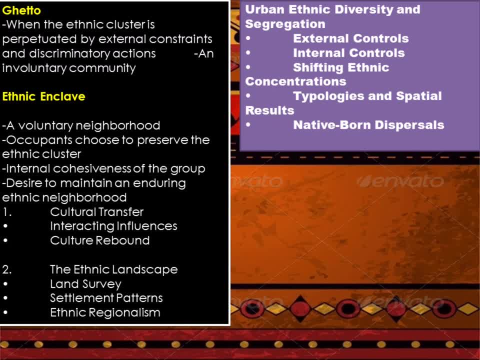 so when we say land survey, it is a system for claiming and allotting land appropriate to cultural needs and traditions, or claiming a land area appropriate to their cultural needs and traditions, cultural needs and traditions. so, uh, that's, uh, the ethnic enclave. now let's go to urban ethnic diversity and segregation. 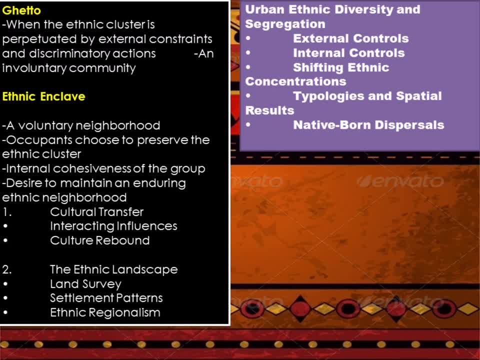 so we have here are three, which is the external controls x internal controls and shifting ethnic. so when we say ethnic controls it is the attitude towards the group. so when an ethnic group is viewed as threatening or blocking tactics used to confine them. tipping point of a community ethnic group. 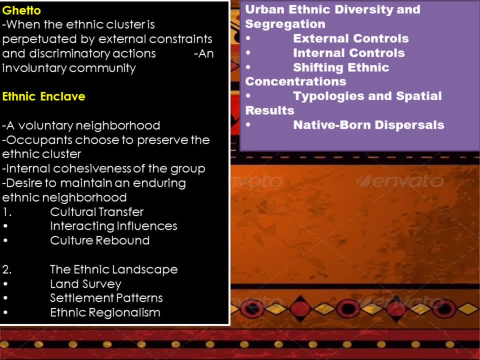 moves into the degree that others move out. so you know it's your attitude towards the group. so next we have internal controls. internal controls is a group's cohesiveness, it is the support. it includes the defense, support and preservation. so the defense limiting exposure to unlimited area.